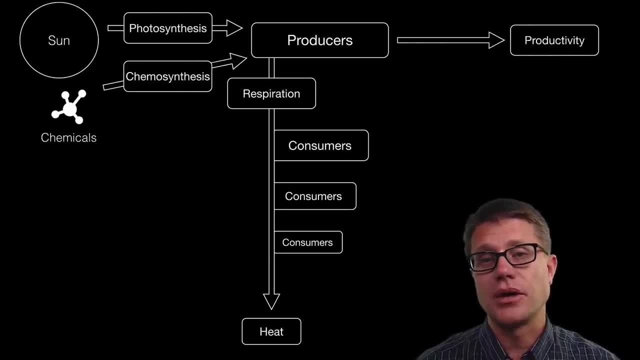 levels. Now we measure the amount of energy that is converted through productivity in one of two ways: Either gross primary productivity or net primary productivity. Gross is the overall amount of energy converted And net is just how much the plant gets after it used some of the energy for respiration. Now each of the levels within this food chain is going. 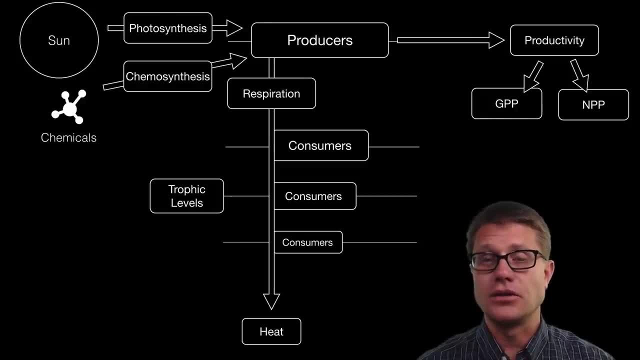 to be a trophic level And we are losing energy along the way, And so a good way to measure this is using an ecological pyramid. We can measure the efficiency, in other words, how much energy makes it to the next level. We can measure the energy at each level, Or we 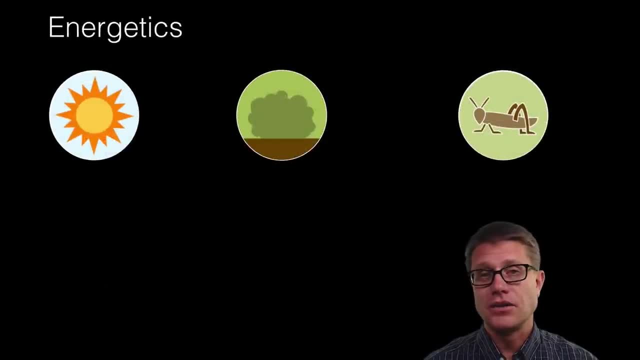 can measure the biomass, How much living material do we have? And so energetics is the study of how energy gets from something like the sun into organisms. What is the most important? first step is going to be photosynthesis. In photosynthesis, we take carbon dioxide in. 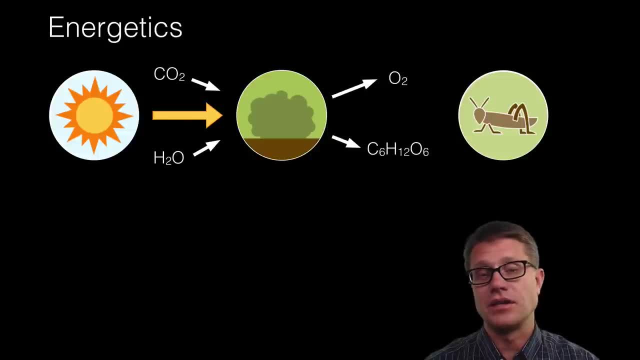 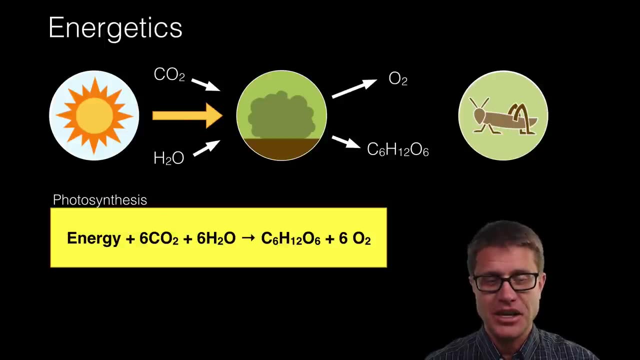 the air, water and the energy in sunlight, and we convert that into oxygen and glucose. If you have not memorized the equation for photosynthesis, now is the time to do it. You should know what is going into the reaction and what is coming out of the reaction, And 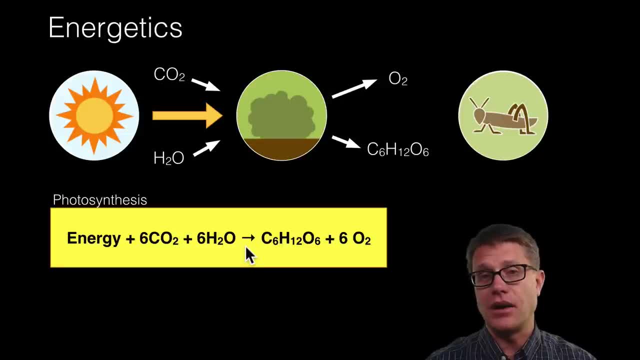 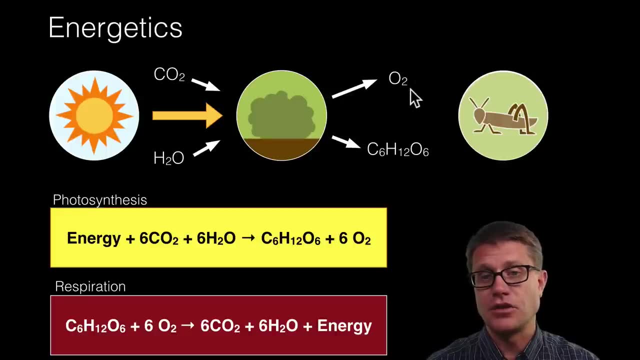 why that is important is we can simply turn the arrow around, and now we have the equation for cellular respiration. So that is what you are doing: You are taking in the oxygen that is produced by plants, Taking in the sugar and you are converting that into carbon. 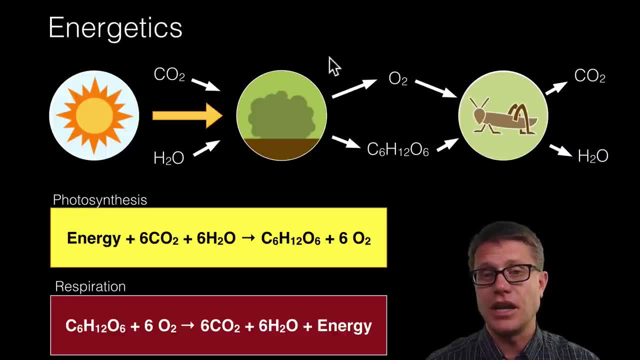 dioxide and water. The nice thing is that this can be recycled again back into plants, And so this is really the way to measure the efficiency of the process. So the first step is really how we take energy, put it in plants, store it in the food, and so we can utilize. 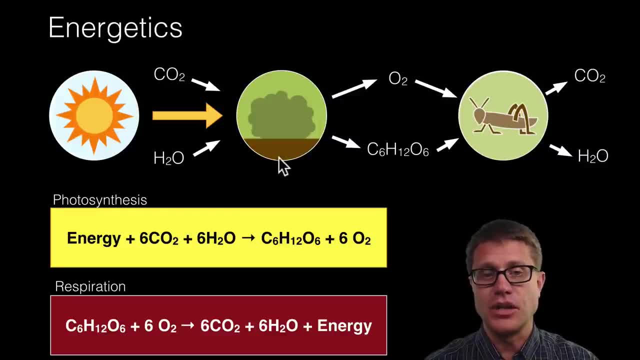 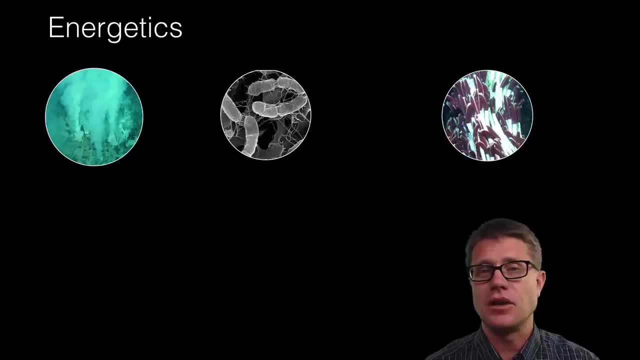 it as well. Now, one major misconception is that plants are doing respiration as well. They are making the sugar for themselves to release that energy. Now, something very similar to photosynthesis is called chemosynthesis, And so if we look down deep in the oceans, 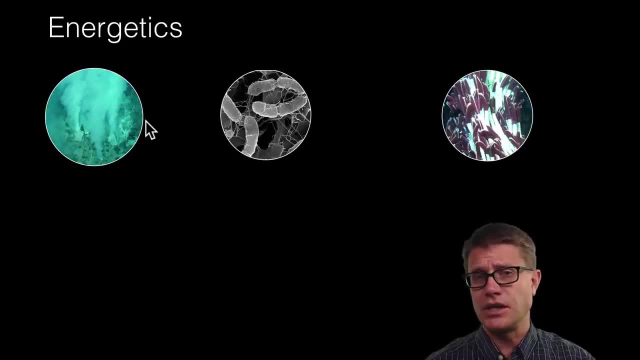 at these hydrothermal vents, we are producing not only heat, but we are producing a chemical hydrogen sulfide. Also, methane can be used this way, And so certain chemosynthetic bacteria- look how similar this is to photosynthesis- can use the energy in the bonds of the hydrogen. 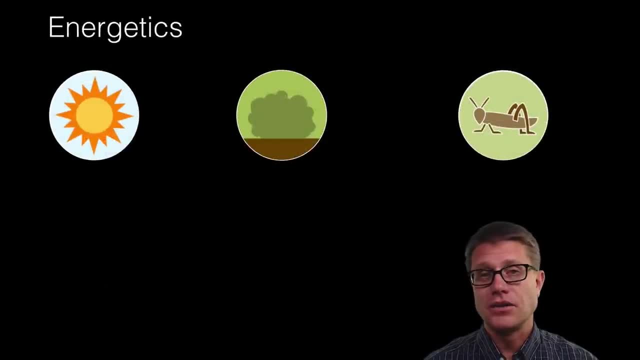 can measure the biomass, How much living material do we have? And so energetics is the study of how energy gets from something like the sun into organisms. What is the most important? first step is going to be photosynthesis. In photosynthesis, we take carbon dioxide in. 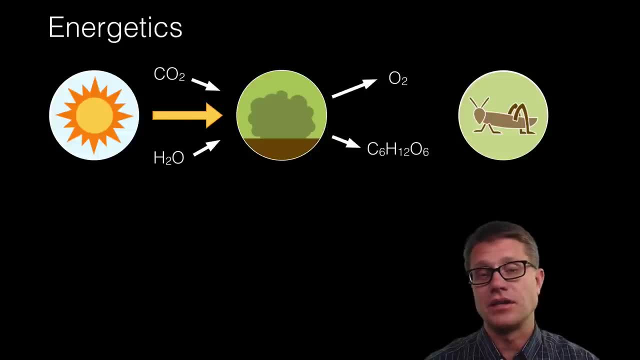 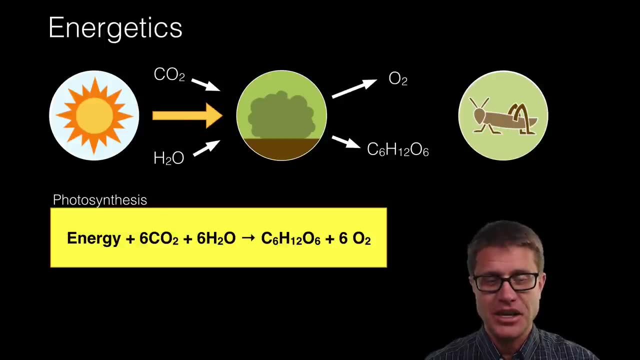 the air, water and the energy in sunlight, and we convert that into oxygen and glucose. If you have not memorized the equation for photosynthesis, now is the time to do it. You should know what is going into the reaction and what is coming out of the reaction, And 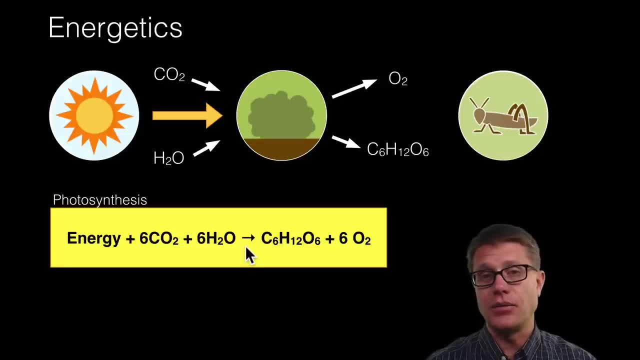 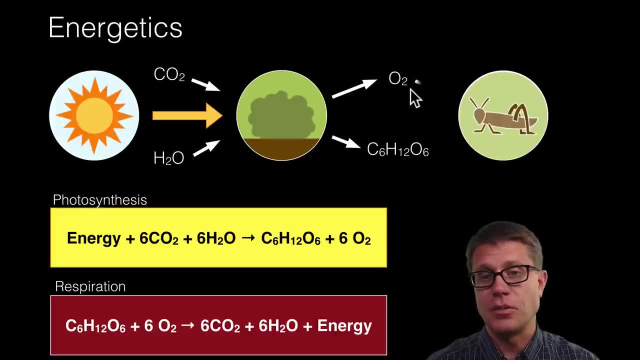 why that is important is we can simply turn the arrow around, and now we have the equation for cellular respiration. So that is what you are doing: You are taking in the oxygen that is produced by plants, taking in the sugar and you are converting that into carbon. 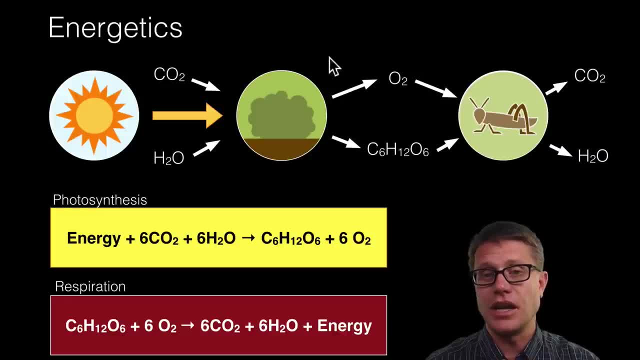 dioxide and water. The nice thing is that this can be recycled again back into plants, And so this is really how we take energy, put it in plants, store it in the food, and so we can utilize it as well. Now, one major misconception is that plants are doing respiration as well. They 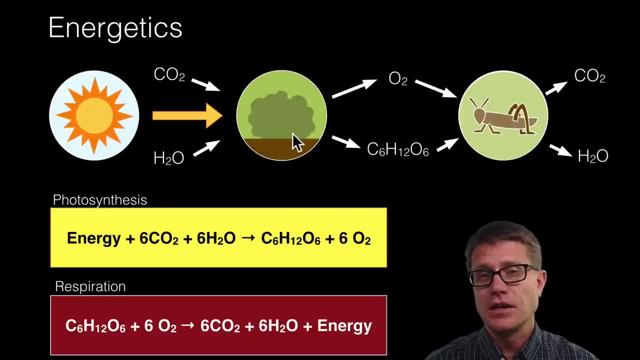 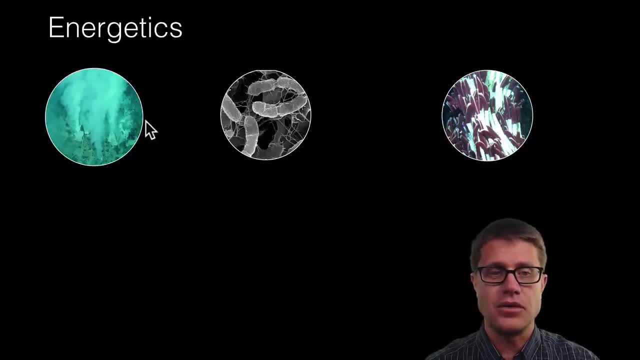 are making the sugar for themselves to release that energy. Now, something very similar to photosynthesis is called chemosynthesis, And so if we look down deep in the oceans, at these hydrothermal vents, we are producing not only heat, but we are producing a chemical hydrogen. 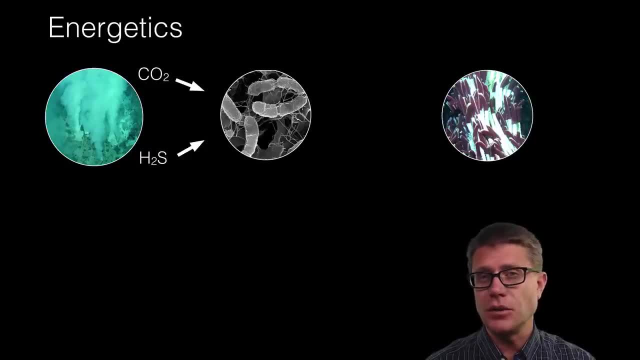 sulfide. Also, methane can be used this way, And so certain chemosynthetic bacteria- look how similar this is to photosynthesis- can use the energy in the bonds of the hydrogen sulfide to make glucose. They release water and then sulfur, And so the equation looks: 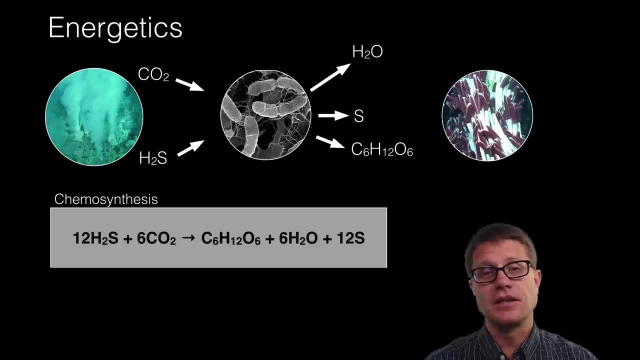 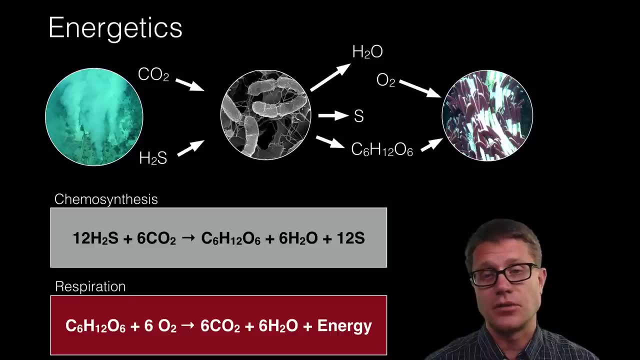 very similar to photosynthesis. Now what happens is things living around. the chemosynthetic bacteria can take in that glucose and they can use oxygen to do cellular respiration, And so we have a totally different system. It is built on the energy of the chemosynthetic. 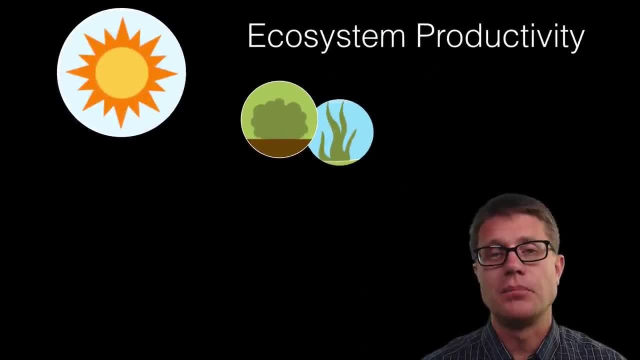 bacteria inside the chemicals. So no matter where the energy comes from, we can measure the amount that gets into the producers using productivity. Now the bad news is that hardly any of that energy actually gets into the plant. 99% is going to move through it bounce. 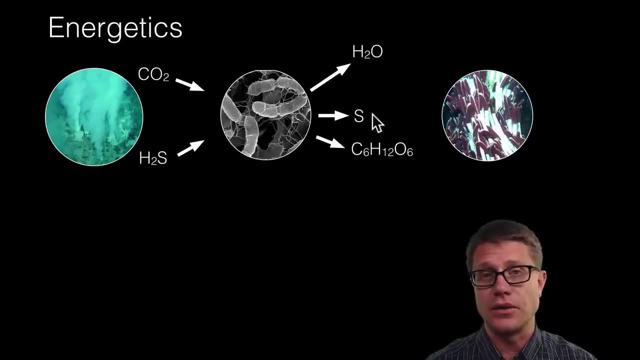 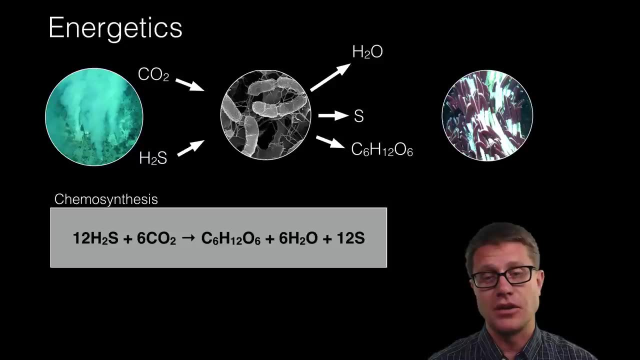 sulfide to make glucose, They release water and then sulfur, And so the equation looks very similar to photosynthesis. Now what happens is things living around, the chemosynthetic bacteria can take in that glucose and they can use oxygen to do cellular respiration. 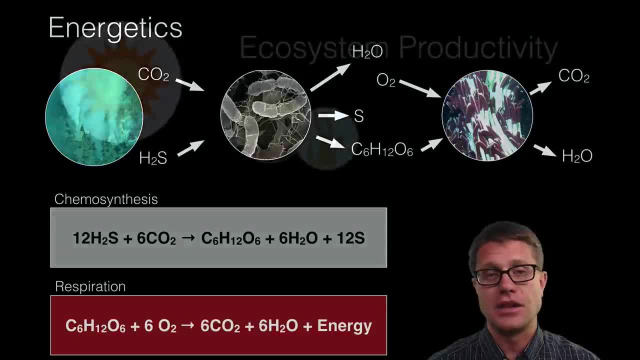 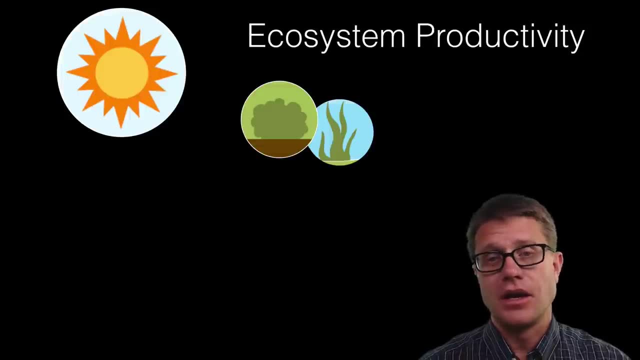 And so we have a totally different system. It is built on the energy inside the chemicals. So no matter where the energy comes from, we can measure the amount that gets released. We can measure the amount that gets into the producers using productivity. Now the bad. 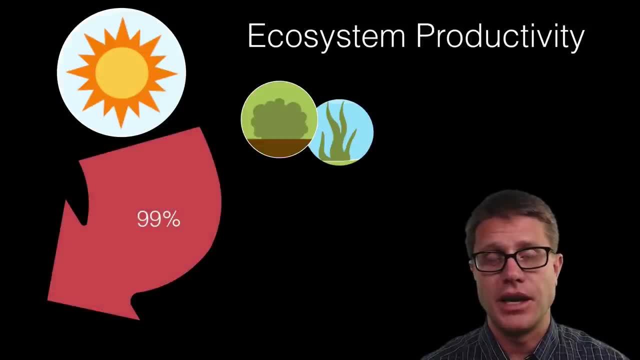 news is that hardly any of that energy actually gets into the plant. 99% is going to move through it, Bounce off of it. The plant does not get it. Only 1% actually goes into the producer And we call that the gross primary productivity. It is the amount of energy that 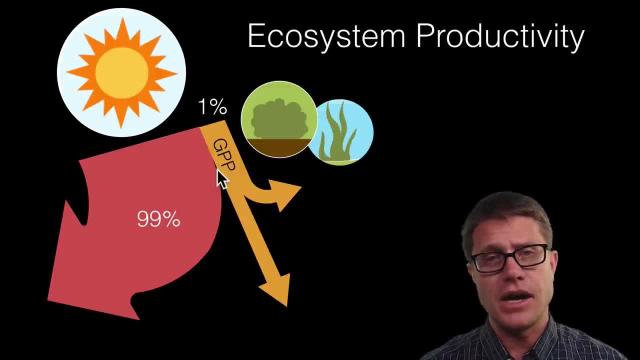 the plant actually gets. Now, what is the plant going to do? It has to survive, And so it is doing respiration. That is where most of the energy goes, And a small percent of it goes to what is called the net production, And that is where most of the energy goes. 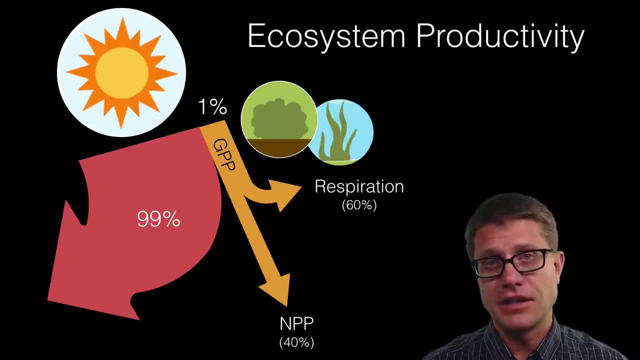 The net primary productivity. That is the amount that the plant gets if we subtract the amount that it used for respiration. So the bad news: not much energy goes into the producers. What is the good news? There is so much energy contained within the sun. If 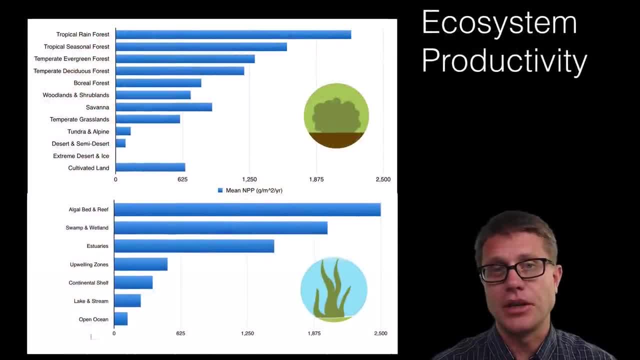 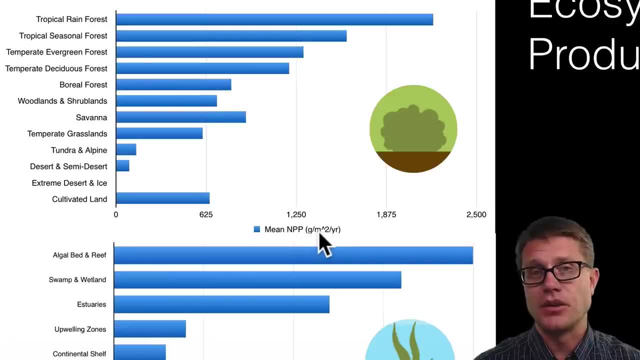 we look at the productivity on our planet, we could compare different terrestrial and aquatic biomes, all the way from the tropical rainforest, which has high productivity. we are measuring that as the amount of material per meter squared per year all the way down to something like a desert. It is not very productive at all. What is interesting is: 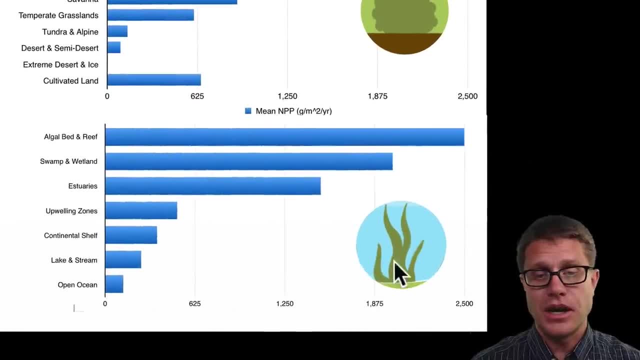 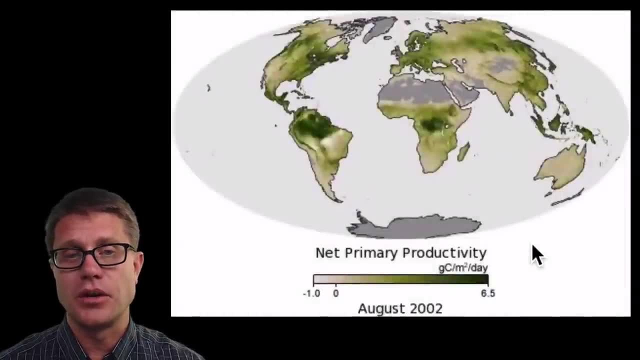 that the amount of energy that we are producing actually does not produce that much. We could compare that to aquatic systems like coral. reefs are incredibly productive. We could even look at how it changes over time. So this is net primary productivity. So this is terrestrial on land. And watch what happens as it changes over an 11 year period of time. 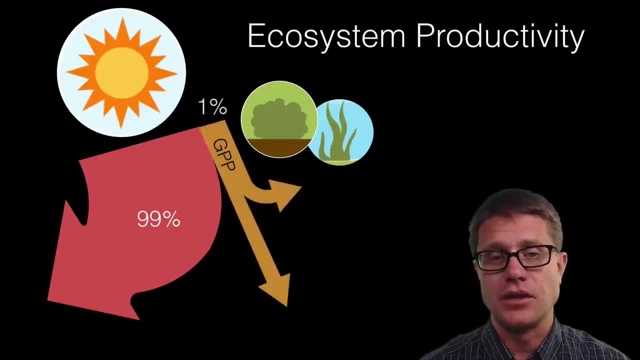 off of it. The plant does not get it. Only 1% actually goes into the producer, And we call that the gross primary productivity. It is the amount of energy that the plant actually gets. Now what is the plant going to do? It has to survive, And so it is doing. 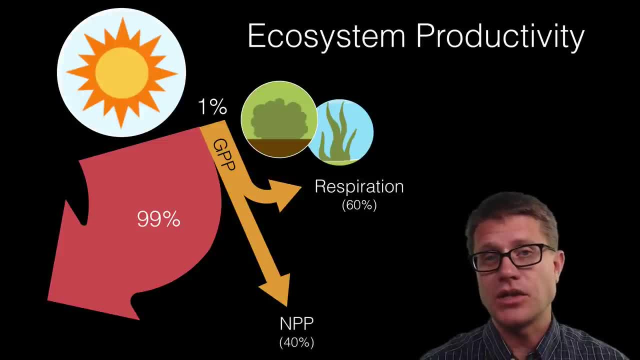 respiration. That is where most of the energy is going to go, And that is where most of the energy goes, And a small percent of it goes to what is called the net primary productivity. That is the amount that the plant gets if we subtract the amount that it used for respiration. 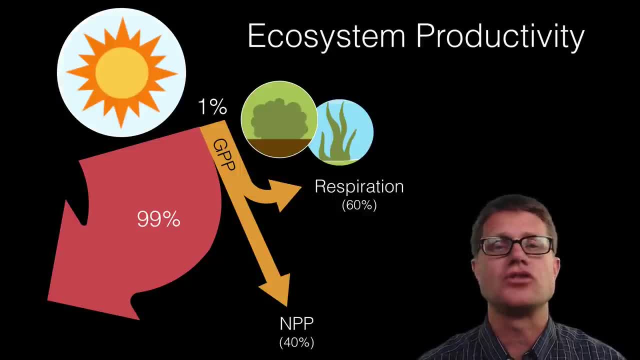 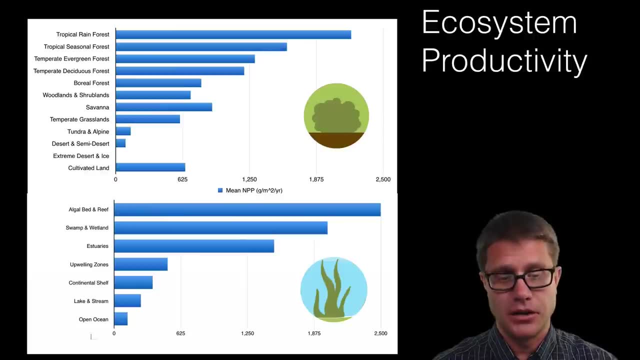 So the bad news: not much energy goes into the producers. What is the good news? There is so much energy contained within the sun. If we look at the productivity on our planet, we could compare different terrestrial and aquatic biomes, all the way from the tropical. 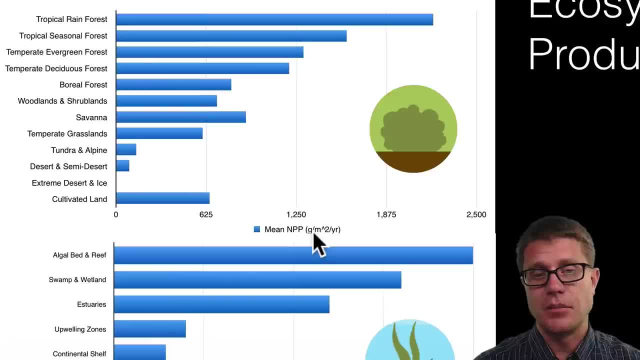 rain forest, which has high productivity. We are measuring that as the amount of material per meter squared per year, All the way down to something like a desert, And that is the amount of material per meter squared per year. So we are measuring that as the amount. 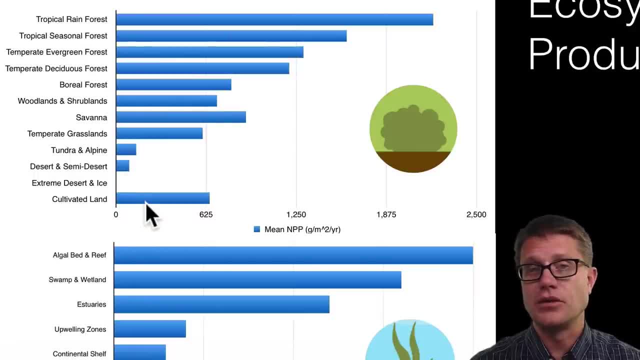 of material per meter squared per year All the way down to something like a desert. It is not very productive at all. What is interesting is that cultivated land actually does not produce that much. We could compare that to aquatic systems like coral reefs are. 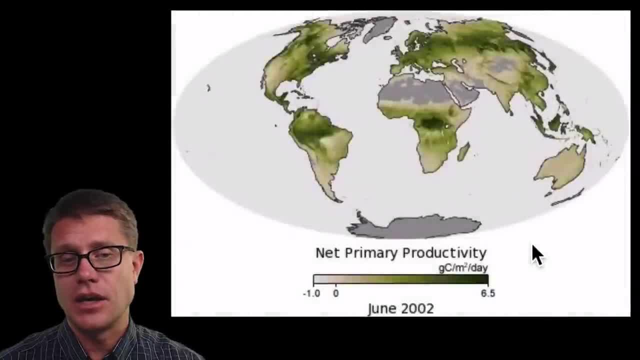 incredibly productive. We could even look at how it changes over time. So this is net primary productivity. So this is terrestrial on land And watch what happens as it changes over an 11 year period of time. You can see it is just moving back and forth. It is moving. 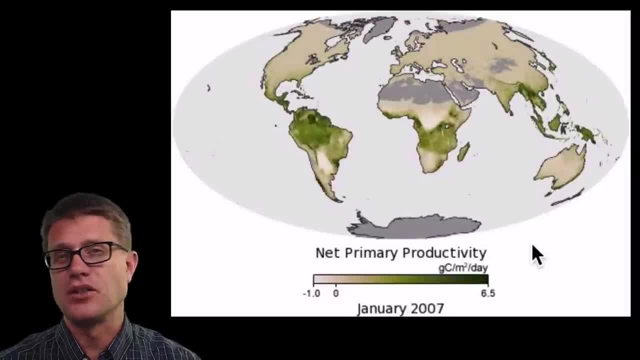 from the southern hemisphere to the northern hemisphere. You can see there is no production in areas where we have massive deserts. But what is causing that change is simply going to be the seasons. During the summer we are going to have way more production where there is way more sunlight, And so an accurate 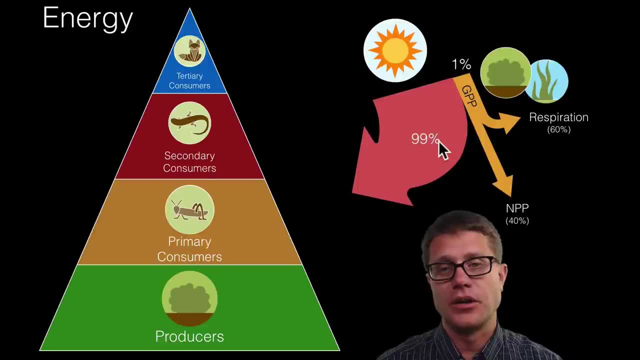 model of measuring how energy is used is an ecological pyramid like this, And so what we are really looking at here is the net primary productivity, The amount at this level, And so if we start here with the producers, let's say that that small percent is actually 100%. 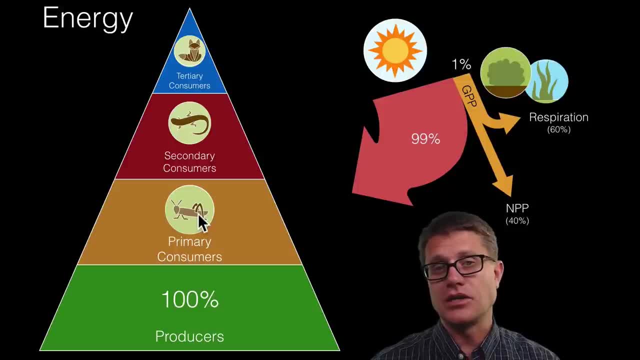 What percent goes to the next level? Well, we are losing energy at each level, And that is because the organism has to survive. It does respiration, And so we are losing heat at each level. And so, in general, of that 100% that the producers get, only 10% goes to the next level. What percent of this goes? 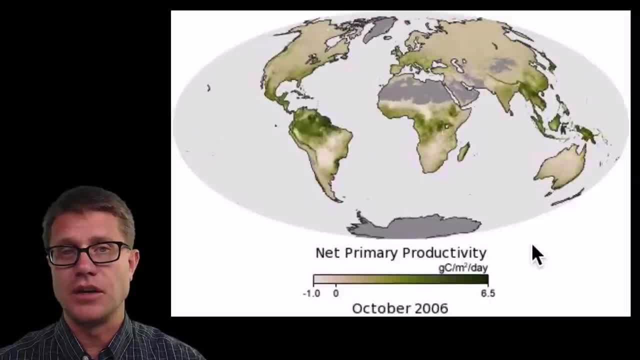 You can see it is just moving back and forth. It is moving from the southern hemisphere to the northern hemisphere. You can see there is no production in areas where we have massive deserts. But what is causing that change is simply going to be the seasons During the 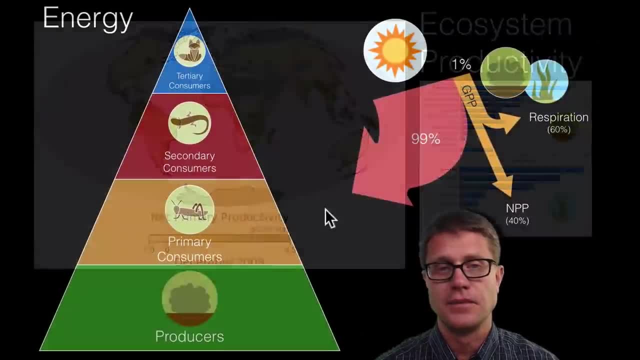 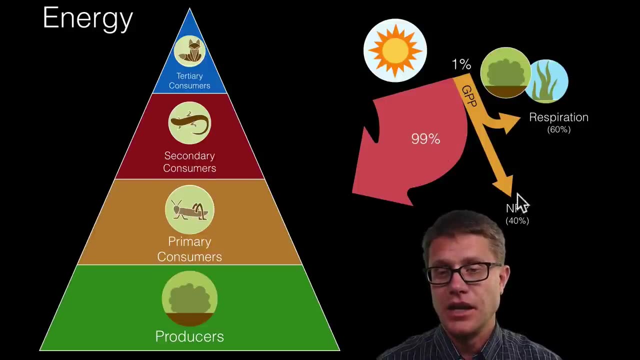 summer we are going to have way more production where there is way more sunlight, And so an accurate model of measuring how energy is used is an ecological pyramid like this, And so what we are really looking at here is the net primary productivity, the amount. 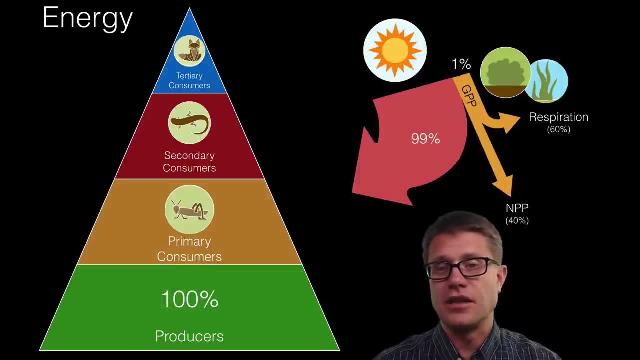 at this level. And so if we start here with the producers, let's say that that small percent is actually 100%. What percentage goes to the next level? Well, we are losing energy at each level, And that is because the organism has to survive. It does respiration, And so we are losing heat at each level And so, in general, if we were a tall virus, we are losing energy at each level, And so, individually, the net primary chop can effectively fall in here In terms of explanations if specific populations, we are at least rid of an individual. 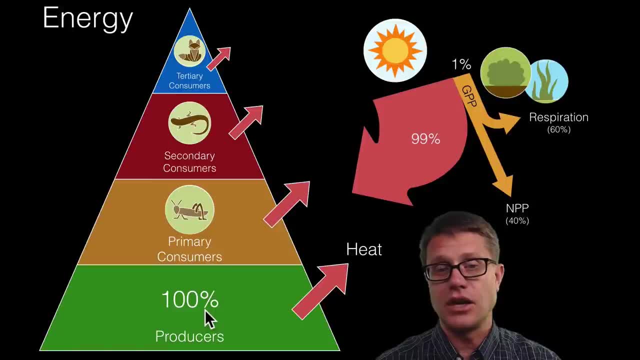 vitamin B or force, etc. But all these measurements you can take out In the Russian. in general, of that 100% that the producers get, only 10% goes to the next level. What percent of this goes to the next level? 10% of that. So now we are down to 1%, And what? 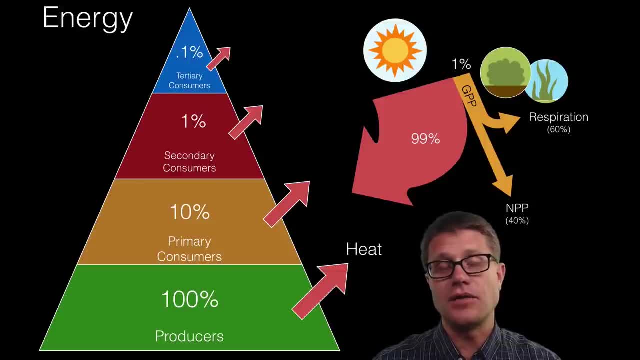 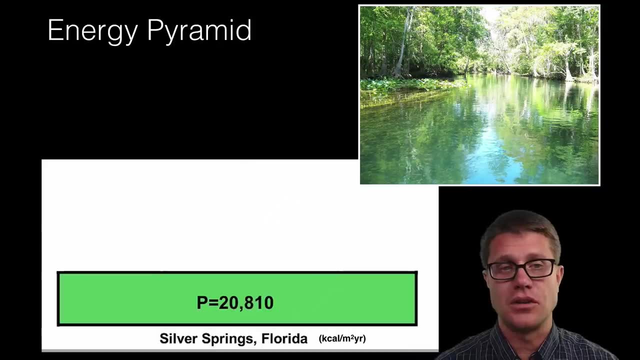 about the next level, 10% of that, And so we are losing a huge amount of energy at each step along the way, And that is going to be why we have way less tertiary consumers than we are going to have producers in an area. A good way to study this is using an energy. 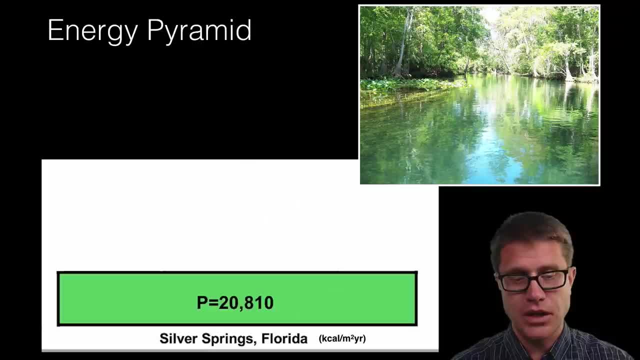 pyramid, And let's look at an actual energy pyramid from Silver Springs, Florida. What we are looking at here is the amount of energy. They are measuring it in kilocals per meter squared per year, And so it is 20,000 kilocals. Now where is the energy found? Just looking. 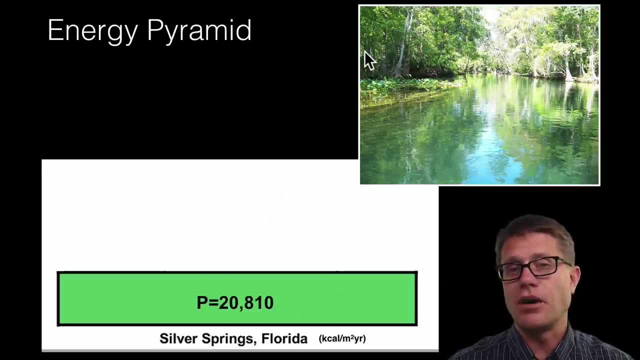 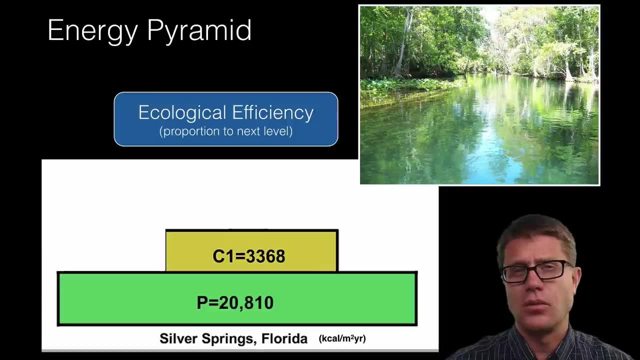 at this picture, it is going to be, for the most part, in these trees. What amount makes it to the next level, to the consumers? Well, when they studied it, it was this amount. So what is the ecological efficiency? What amount made it to the next level? Well, you. 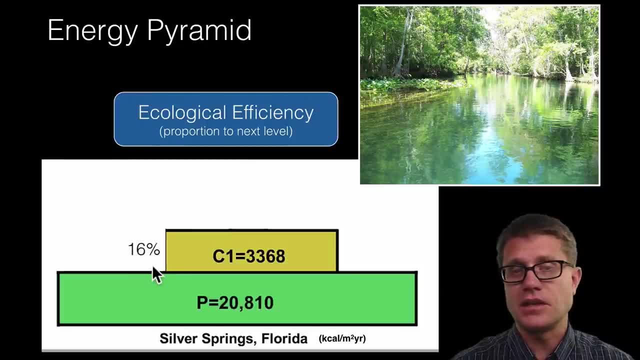 could just take this and divide it by that And we could find that 16% moved to the next level. We could look at the secondary consumers- You can see it is around 10% there- And we could look at the tertiary consumers And 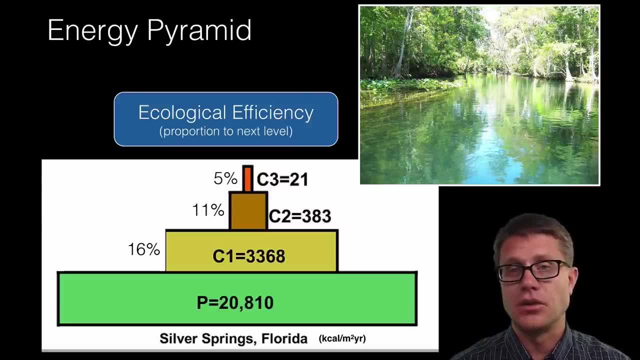 you can see that it is around 5%, And so ecological efficiency is going to be somewhere between 5 and 20%, depending on how efficient that ecosystem is. Now, what are we really missing on this energy diagram are the decomposers. They are going to make use of a lot of that. 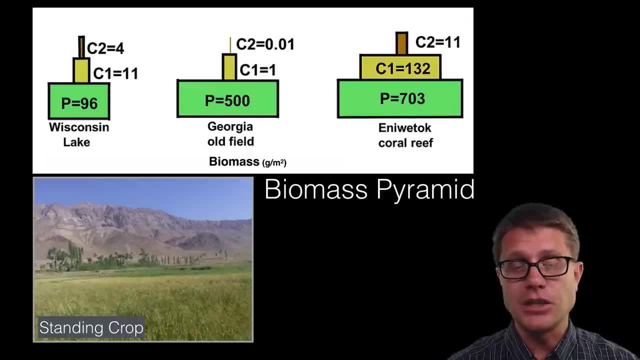 energy as well. Another way to measure it is biomass: Just how much material is made. What is different here is that we do not measure it over a given period of time. We measure what is called standing crop. It is the amount that is there. It is the amount that is there. 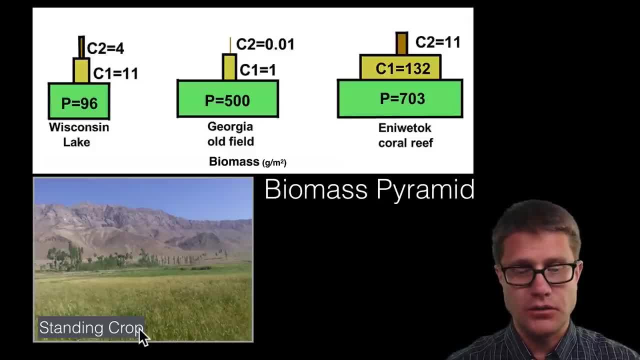 at one point in time. But you can see the same thing occurs If we are looking at a Wisconsin lake or a field or a coral reef. the amount of biomass that we have at the producer level is going to be way more than we have at the levels above it, And so did. 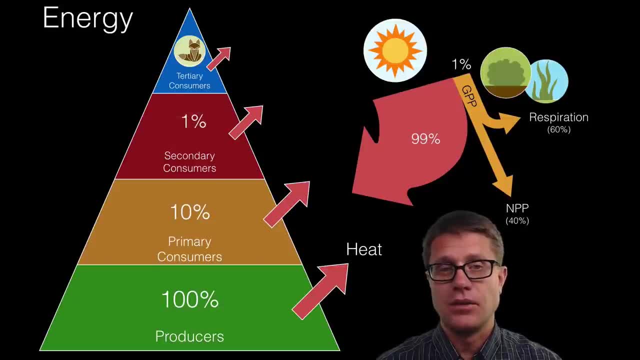 to the next level- 10% of that. So now we are down to 1%. And what about the next level? 10% of that? And so we are losing a huge amount of energy at each step along the way, And 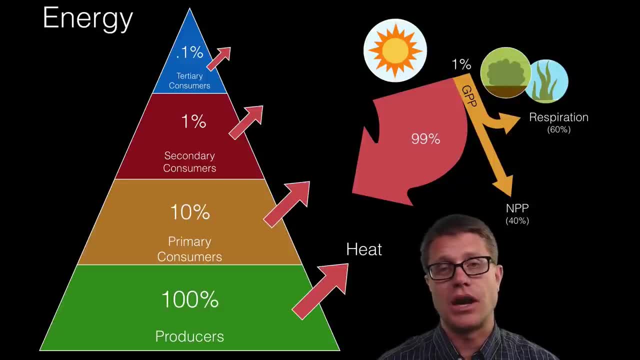 that is going to be why we have way less tertiary consumers than we are going to have producers in an area. A good way to study this is using an energy pyramid, And let's look at an actual energy pyramid from Silverstone. So let's look at Silverstone. So Silverstone is a very 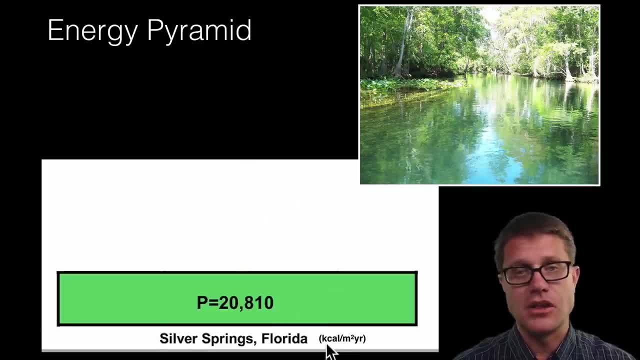 very small city in Silver Springs, Florida. What we are looking at here is the amount of energy. They are measuring it in kilocals per meter squared per year, And so it is 20,000 kilocals. Now where is the energy found? Just looking at this picture, it is going to be. 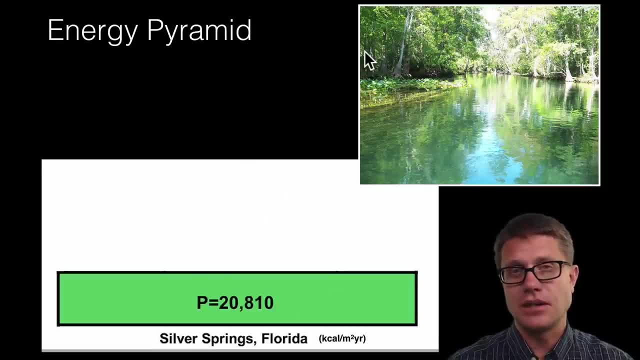 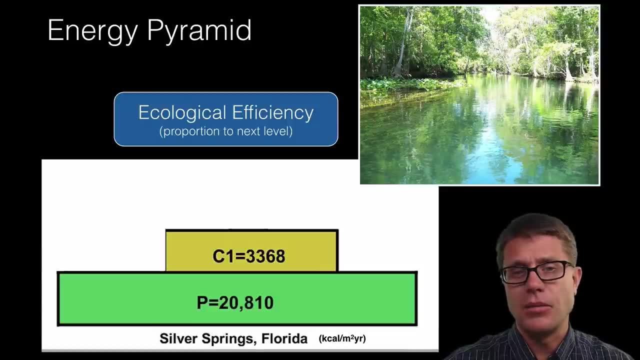 for the most part in these trees. What amount makes it to the next level, to the consumers? Well, when they studied it, it was this amount. So what is the ecological efficiency? What amount made it to the next level? Well, you could just take this and divide it by that. 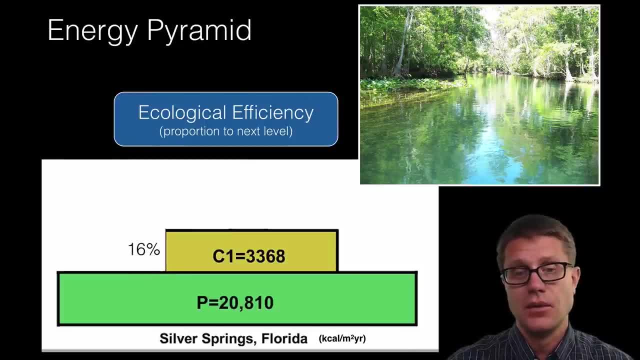 And we could find that 16% moved to the next level. And we could look at the secondary consumers: You can see it is around 10% there. And we could look at the tertiary consumers And you can see that it is around 5% And so ecological. 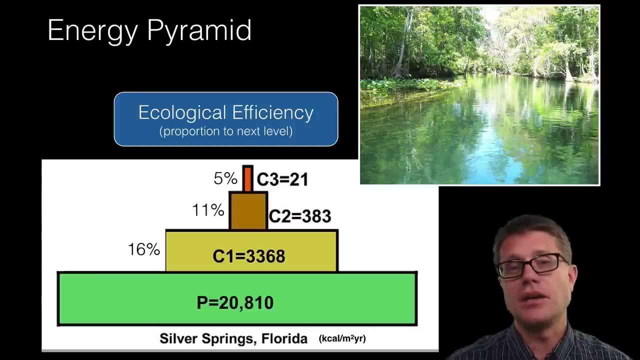 efficiency is going to be somewhere between 5 and 20%, depending on how efficient that ecosystem is. Now, what are we really missing on this energy diagram are the decomposers. They are going to make use of a lot of that energy as well. Another way to measure it. 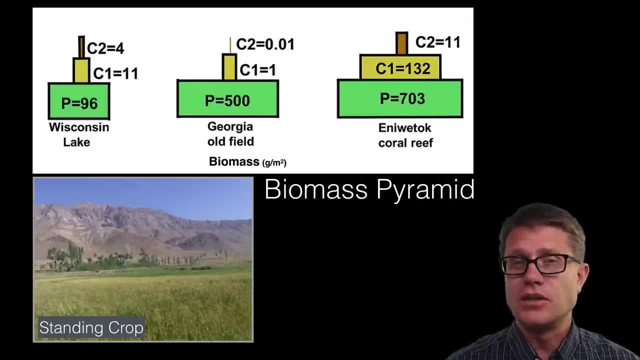 is biomass, Just how much material is made. What is different here is that we do not measure it over a given period of time. We measure what is called standing crop, And what we measure is what is called standing crop, And what we measure is what is called standing. 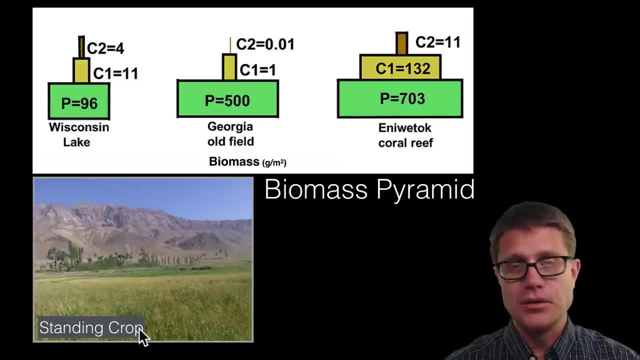 crop. It is the amount that is there at one point in time. But you can see the same thing occurs if we are looking at a Wisconsin lake or a field or a coral reef. The amount of biomass that we have at the producer level is going to be way more than we have at the 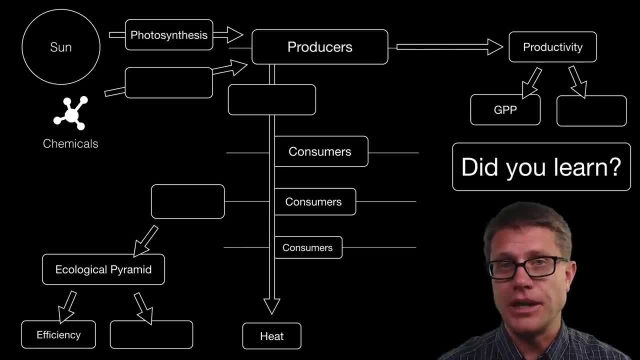 levels above it, And so did you learn the following. Can you fill in all the blanks? Pause the video. If not, I would say that energy comes from chemicals through chemosynthesis to producers. We could measure productivity as gross or net primary productivity. How? 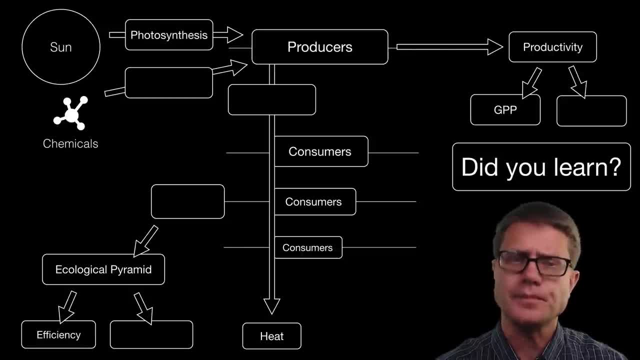 you learn the following. Can you fill in all the blanks? Pause the video. If not, I would say that energy comes from chemicals through chemosynthesis to producers. We could measure productivity as gross or net primary productivity. How do we utilize that energy? This would 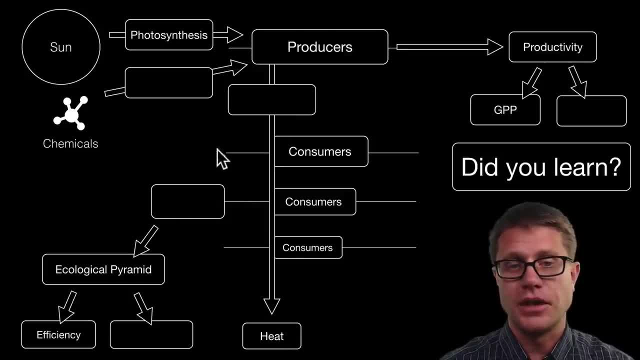 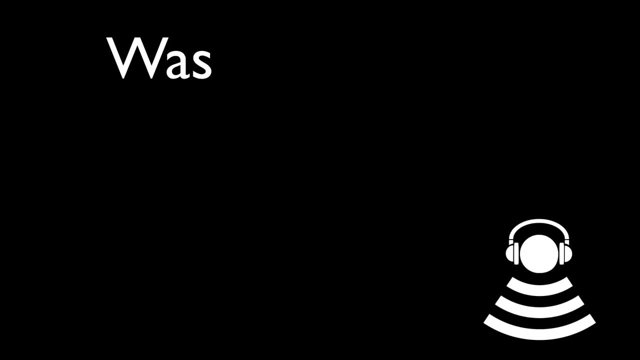 be respiratory Expiration all the way down to heat. We then have the trophic levels. Those are going to be the feeding levels. Ecological pyramids measure efficiency And we can also measure the biomass, And I hope that was helpful.